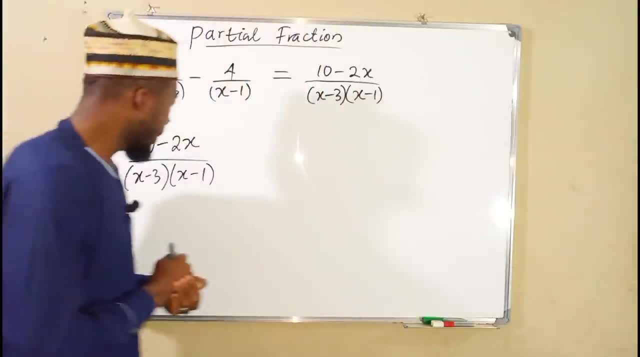 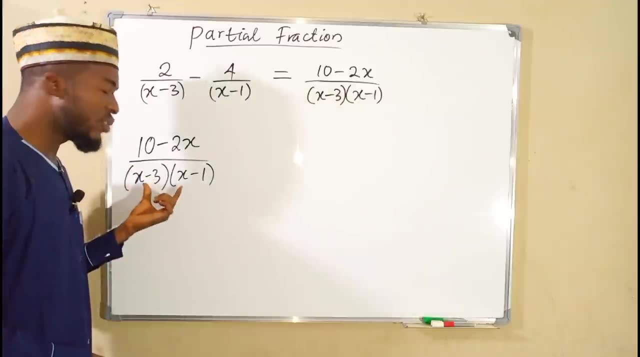 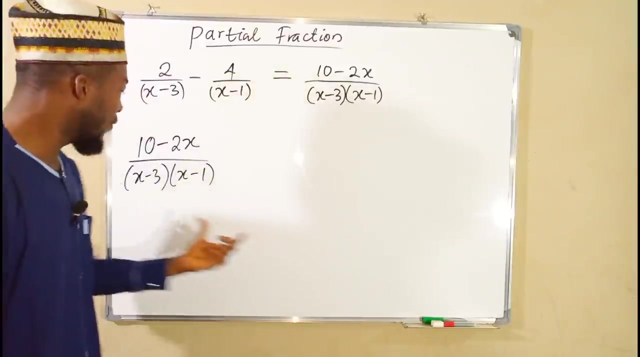 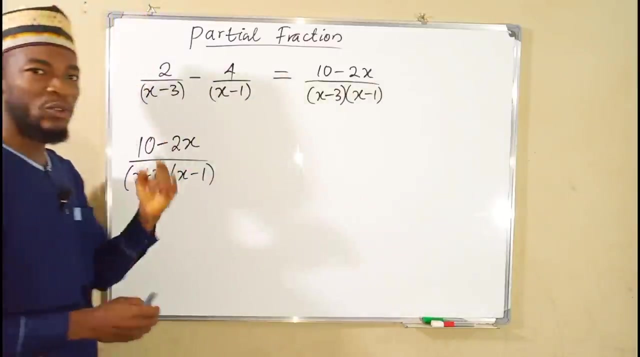 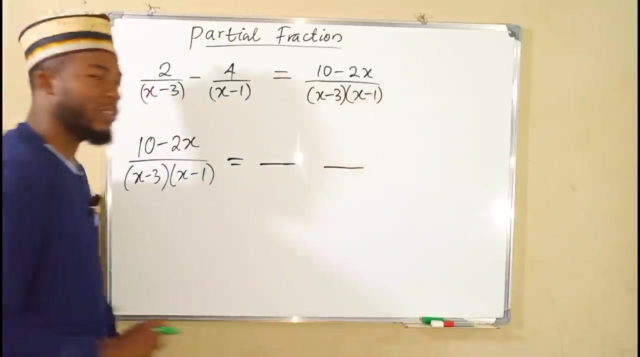 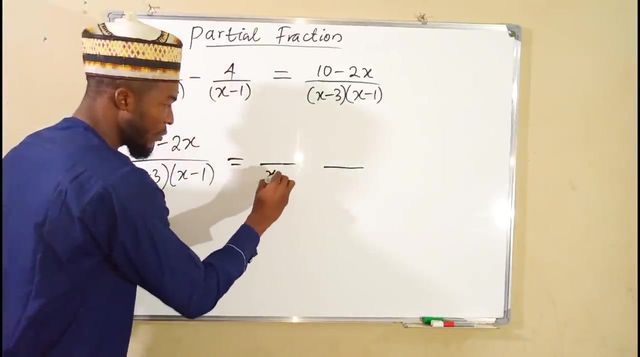 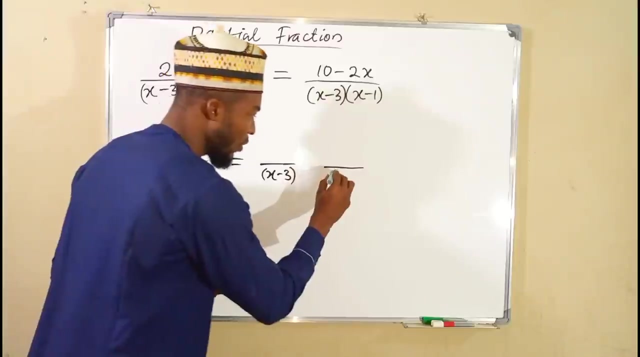 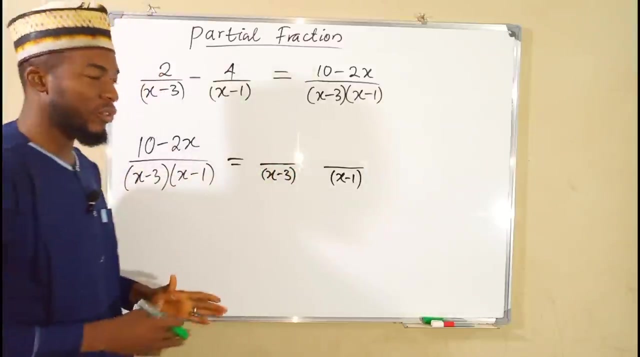 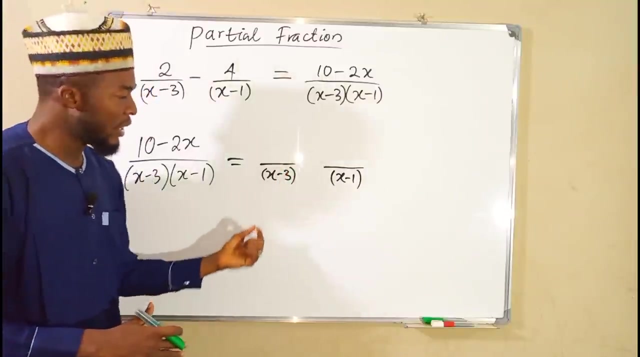 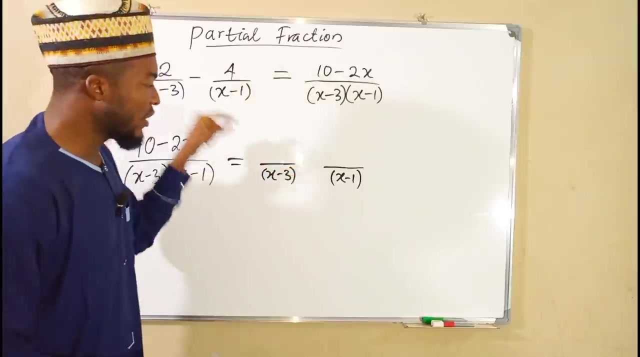 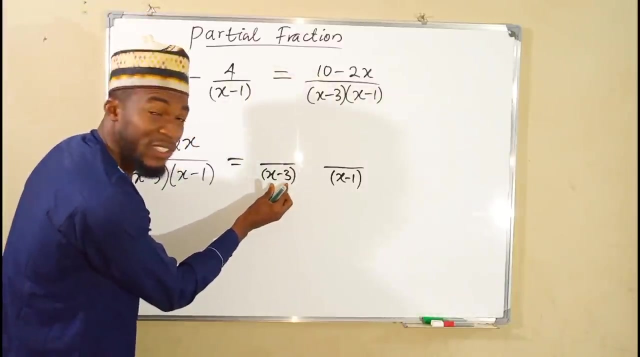 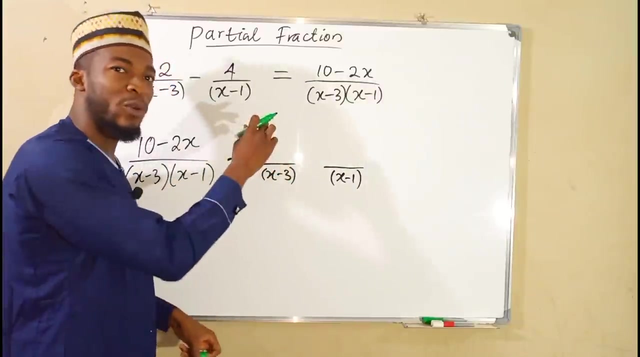 whenever I upload a new content. So whenever you are given a compound fraction to split it into partial fractions, always consider your denominator. The number of factors you have there will determine the number of fractions you are going to obtain. For instance, here that we have just two factors, we are going to obtain two sets of fractions. That's number one. So we are going to obtain two sets of fractions. So the first fraction is going to contain x minus three as its denominator, x minus three, while the second fraction is going to contain x minus one as its denominator, x minus one. Then how can we obtain their corresponding numerators? To obtain their corresponding numerators, you have to examine the nature of these factors. You can see each of these factors are linear factors. So the numerator of each of these fractions is going to be a polynomial of one degree less than the denominator. And you can see the denominator is of the degree one. Therefore, one minus one is zero. Hence, we are going to obtain a constant to the top. We can call that constant A. 1 minus one is zero. Hence, we are going to obtain a constant to the top. We can call that constant A. 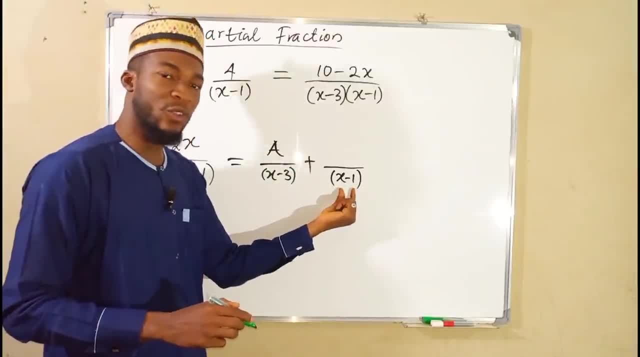 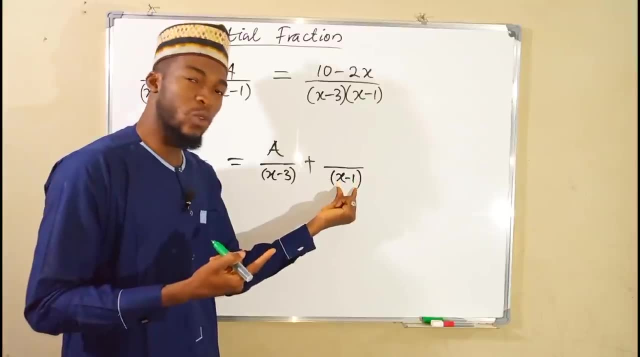 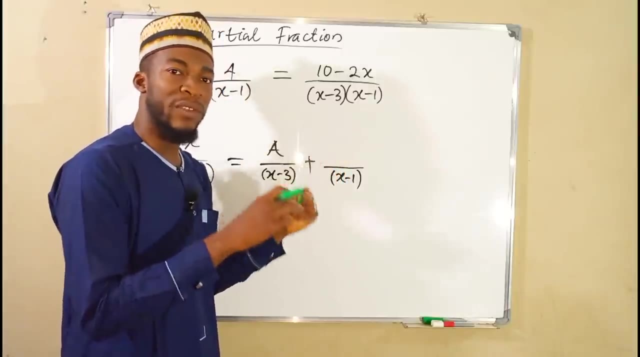 plus the other one it's also a linear factor of degree one so the numerator is going to be a polynomial of one degree less than the denominator one less meaning one minus one is zero hence we have no variable to the top leaving only constant and we call it 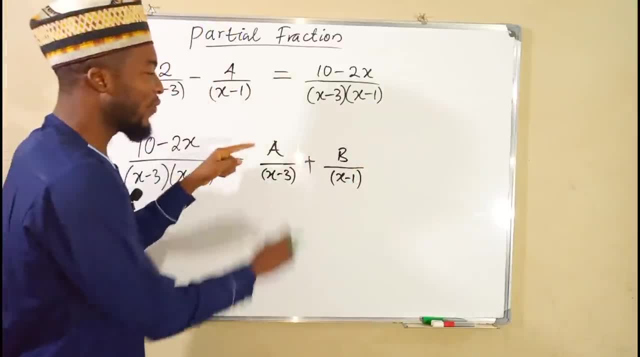 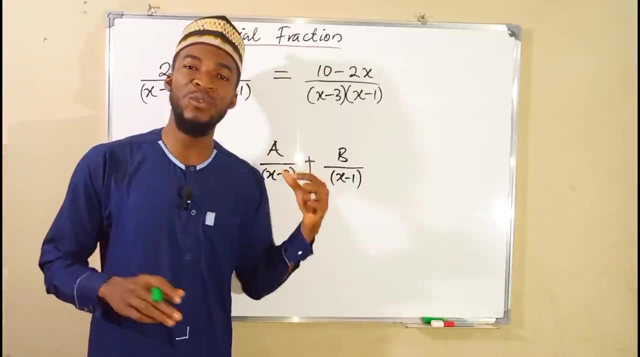 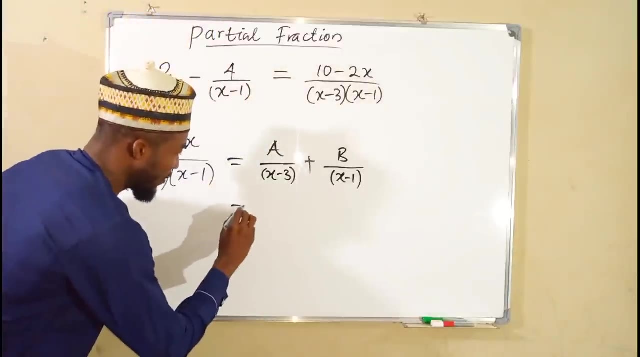 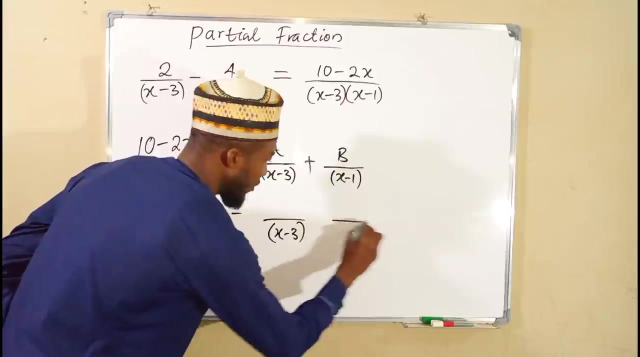 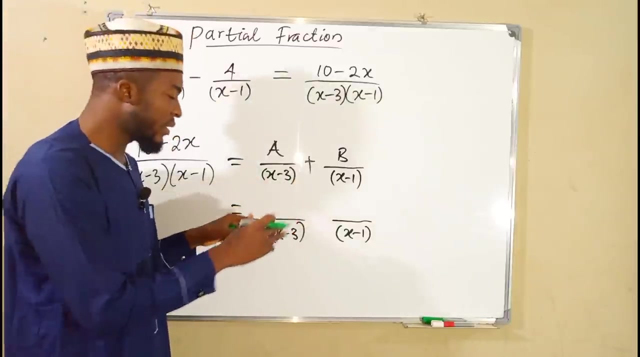 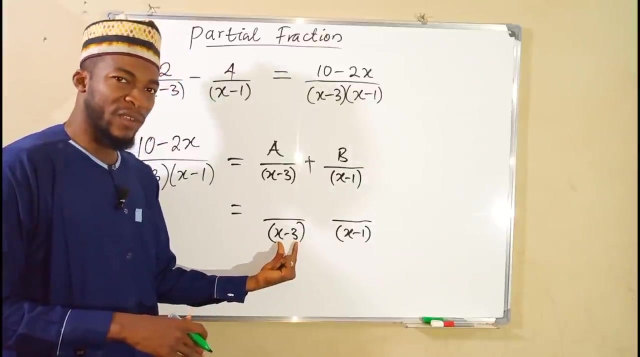 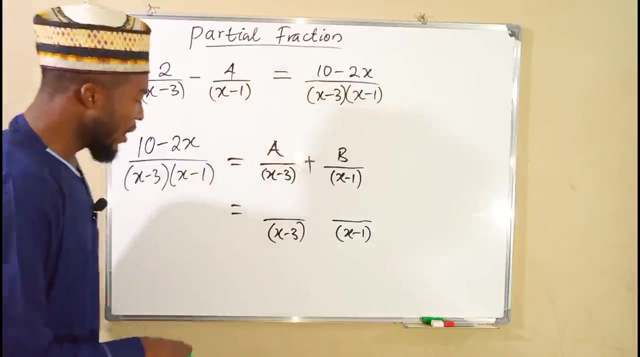 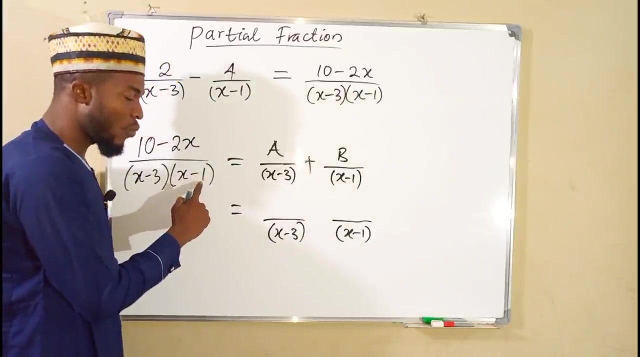 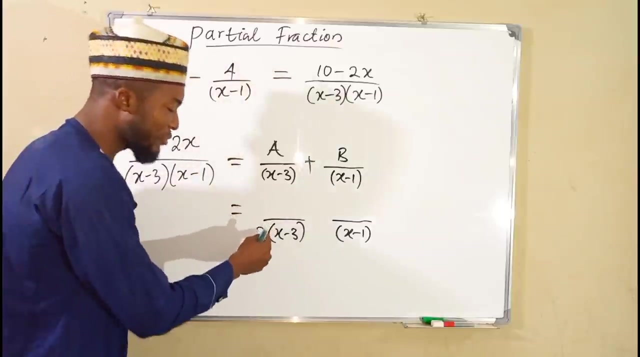 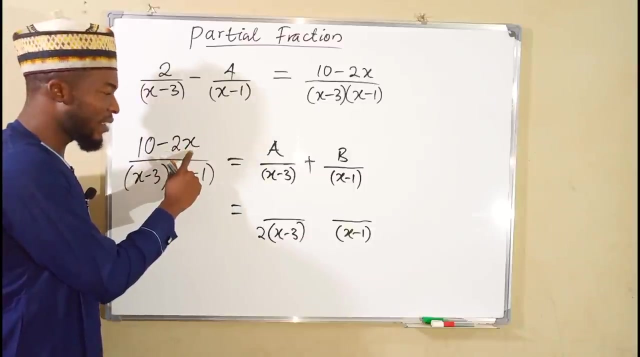 b so now what we are going to do we are going to find the corresponding constants of a and b respectively and there are a couple of ways for which we can find this constant and the first method i'm going to introduce is the cover-up method so this goes like this we have our first fraction x minus three we have our second fraction x minus one now to find their cross-funding constant let us first of all consider this factor which is x minus three we want to transform this factor into zero by setting the value of x to be equal to three because three minus three is zero and hence we are going to substitute that three into the other factor which is x minus one three minus one is two so we have our two here to the bottom and to obtain the top number we are going to substitute that three from our numerator here so we have two times three is six 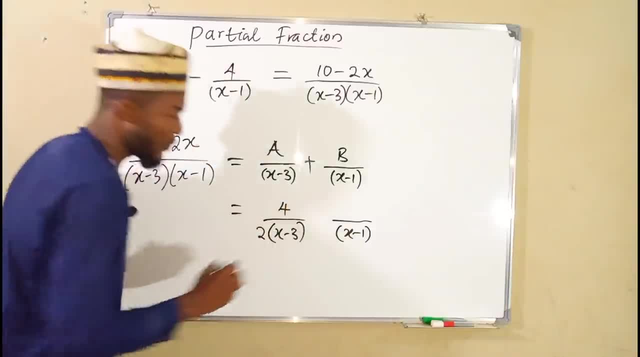 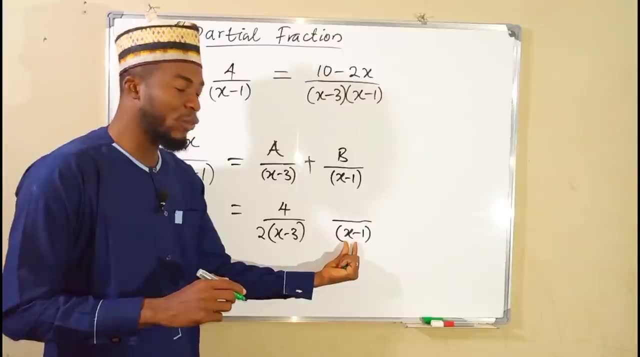 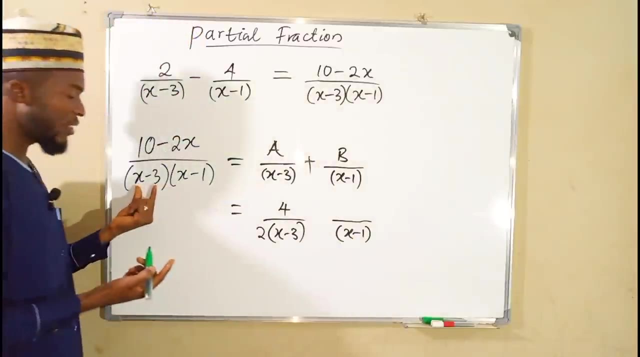 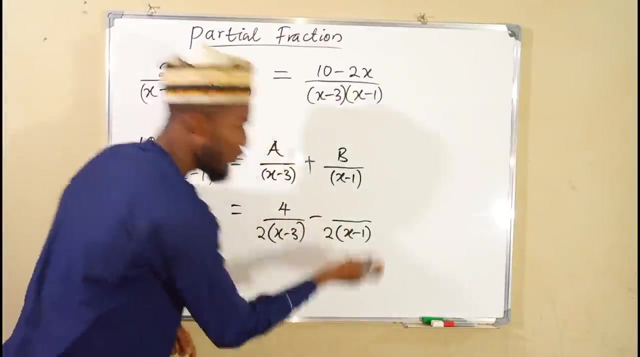 then ten minus six is four so we have four here then the next one we have x minus one we want to set it to be equal to zero by setting the value of x to be equal to one then one minus one is zero hence we are going to substitute that one into the other factor then one minus three is negative two so we have negative we have two to the bottom to obtain the top number we are going to substitute 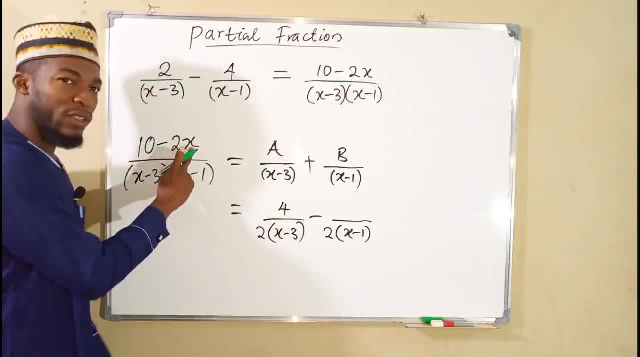 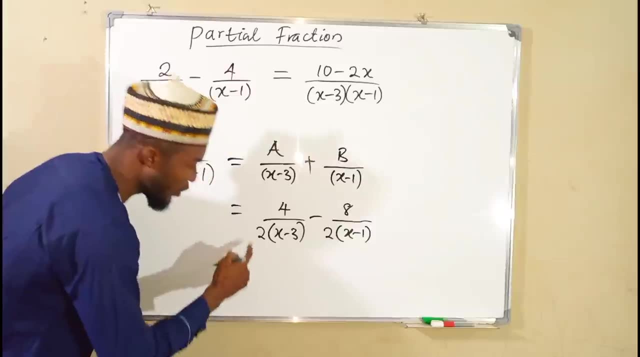 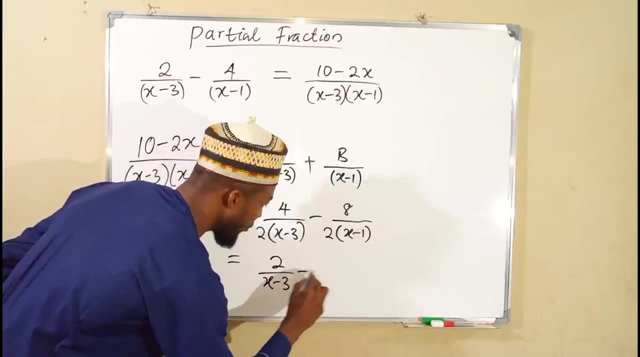 the positive into the bottom order and then we are going to substitute that named after x at contact area our four replace the negative point for x i will actually repeat this so if we have x minus 12 plus two here we have eight so yeah three times two 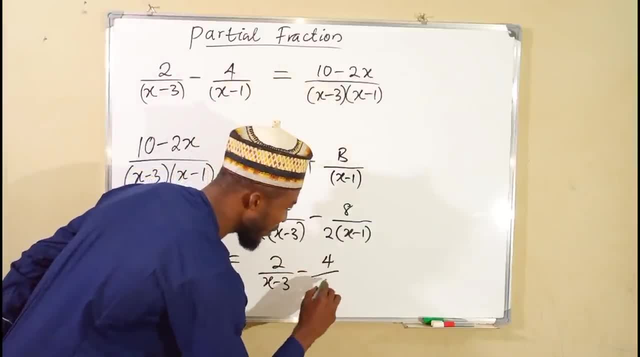 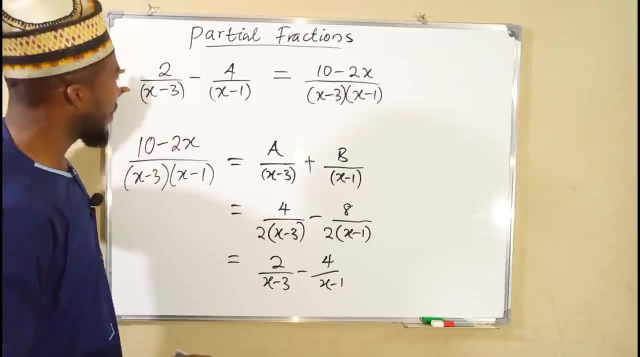 now our nameんumerator here two times one is two then ten minus two is eight so we have here we further simplify we know two can go in to four two times 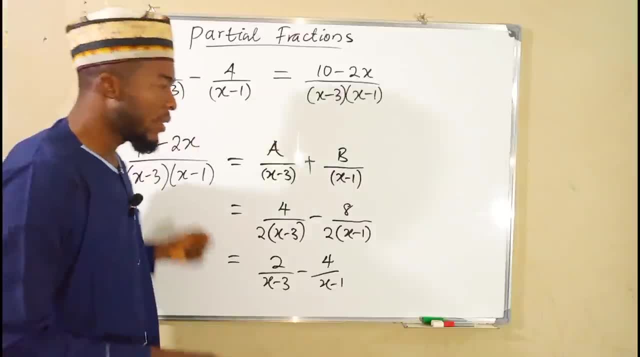 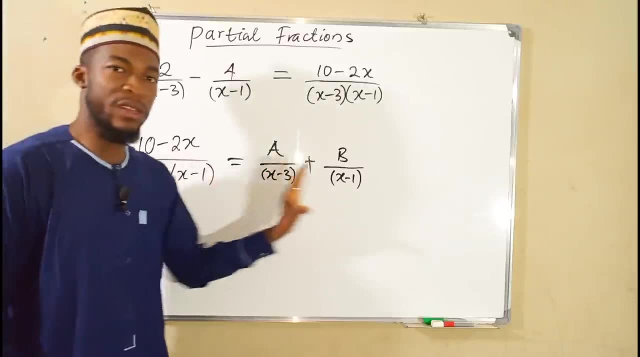 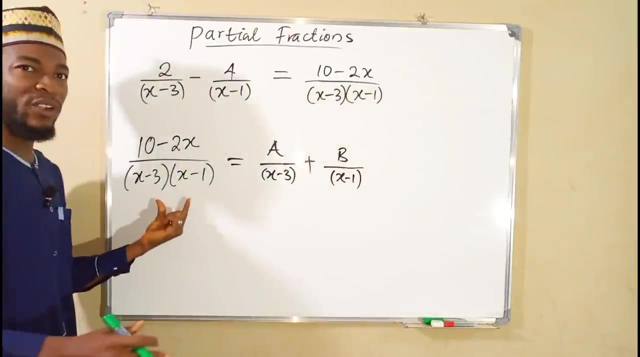 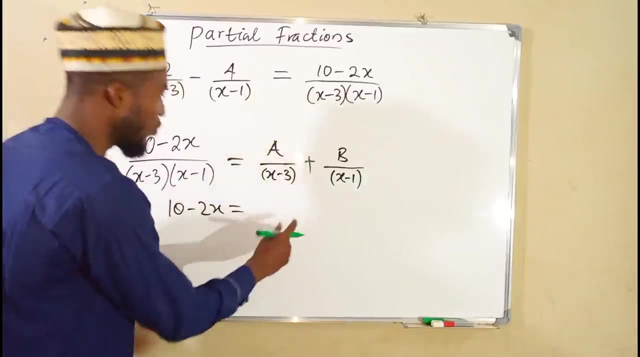 as the initial partial fractions and this is not the only method for which we can find the values of a and B let me show you the next one after making this arrangement we want to clear the fractions you see if we multiply each of these terms by these two factors definitely we are going to clear all fractions by multiplying the left-hand side by these two factors they are going to cancel out leaving only the numerator 10 minus 2 X this is equal to we are 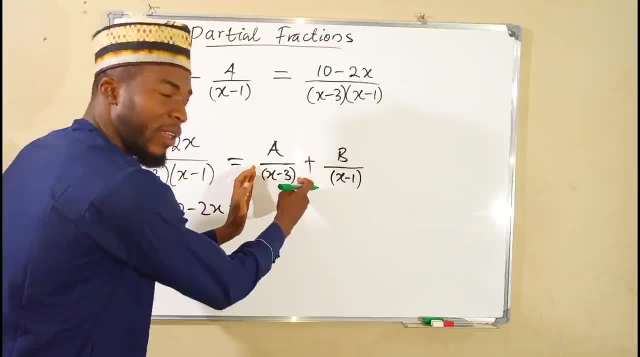 going to multiply this first term from the right hand side with these two 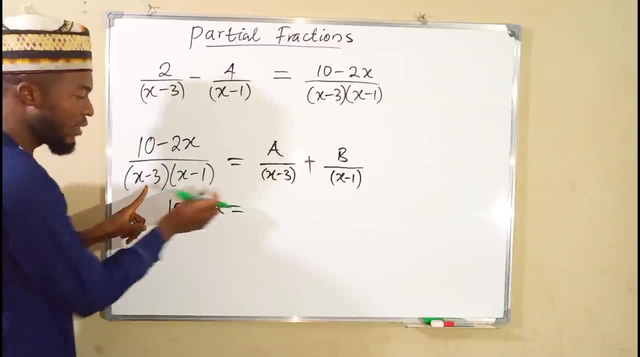 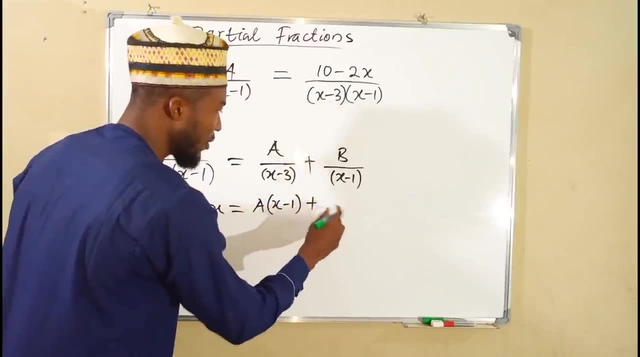 factors definitely this factor will cancel this one leaving only X minus 1 multiplied by a so we have a X minus 1 then plus if you multiply the second 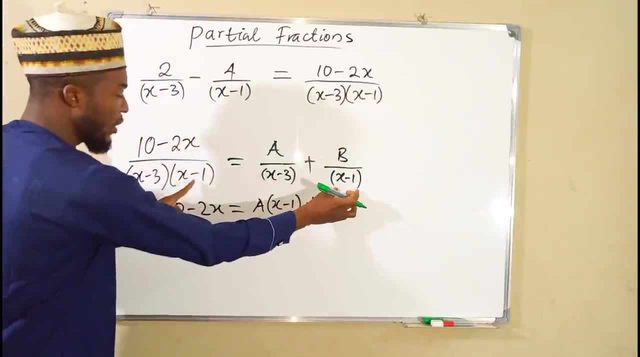 fraction by these two factors this X minus 1 will cancel this X minus 1 leave inside the denominator by the first underwrite so we have a minus 1 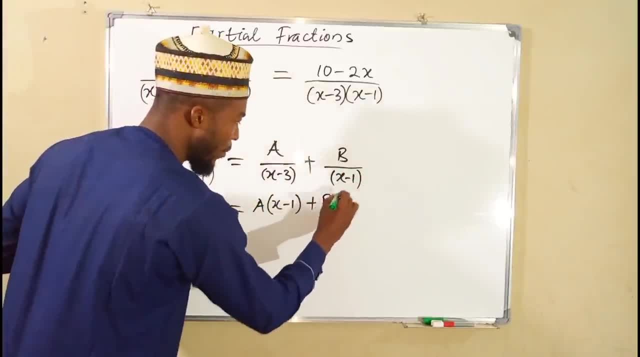 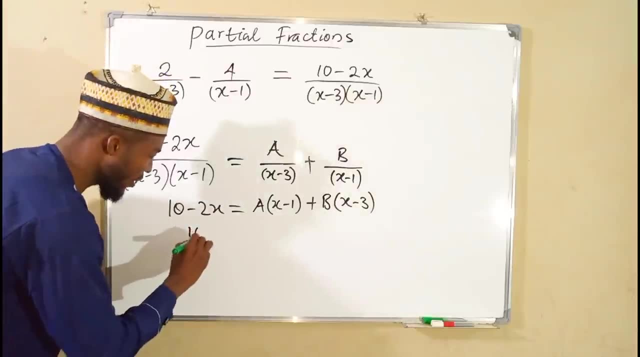 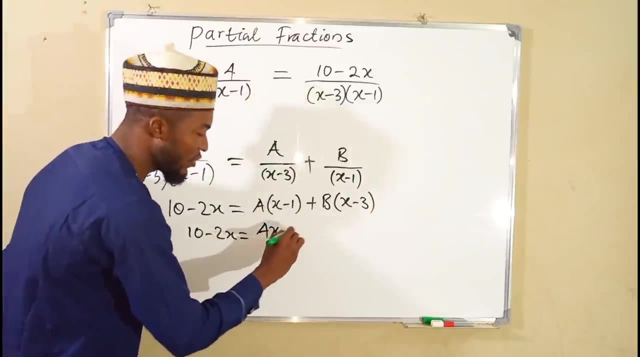 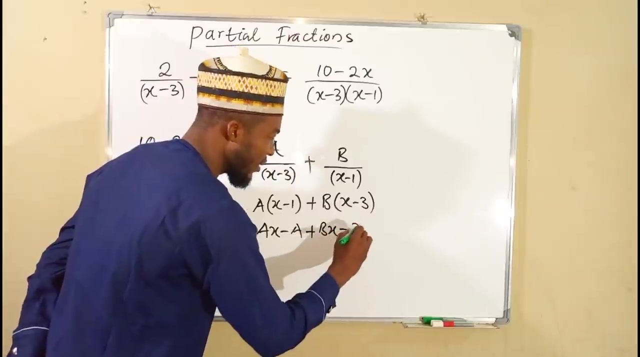 given x minus 3 multiplied by b. Again, we are going to expand each of these brackets. We have 10 minus 2x. This is equal to ax. a times negative 1 is negative a. b times x is bx. b times negative 3 is negative 3b. All those with x, we connect them together. 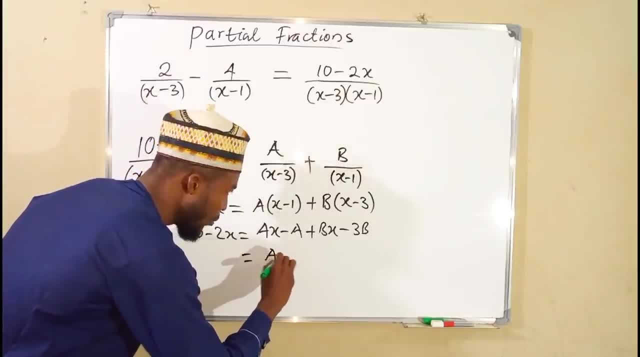 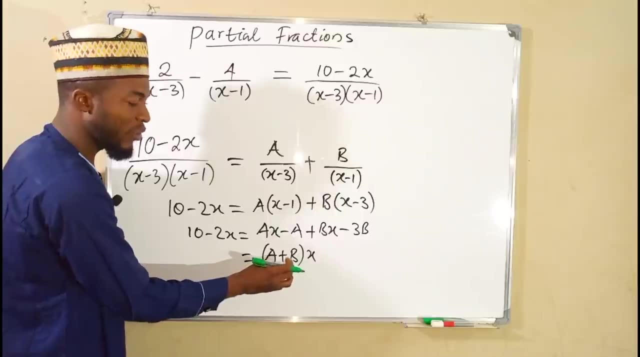 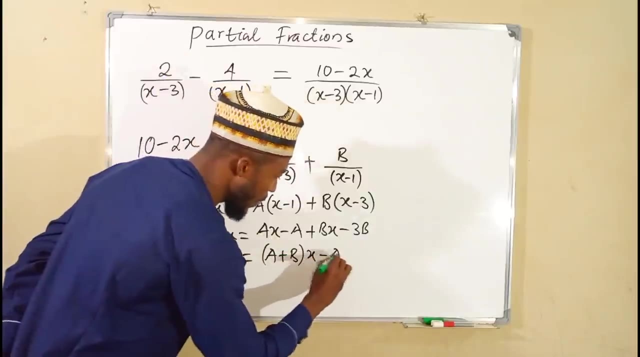 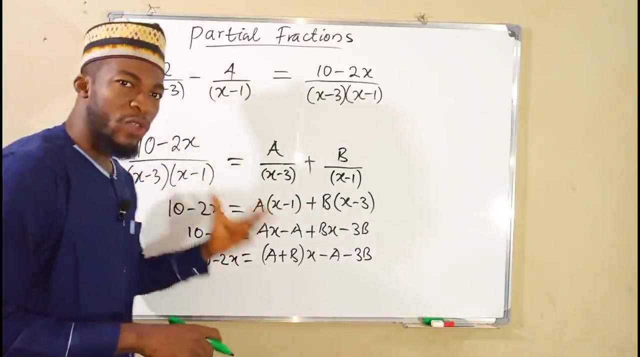 We have a plus b. We can factor the x out because we have ax plus bx. a plus b, I have already factored my x out. Then the other term that does not contain x, we have negative a and we have negative 3b. This is 10 minus 2x. So now we are going to relate their coefficients. 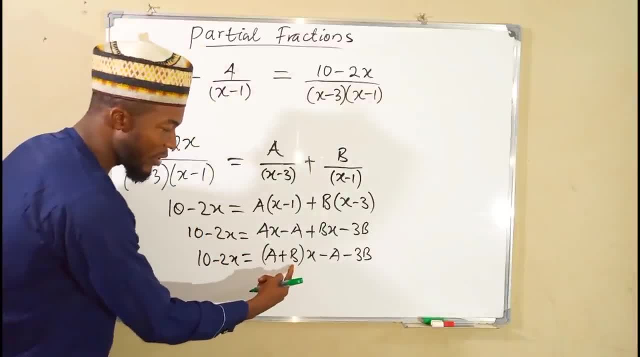 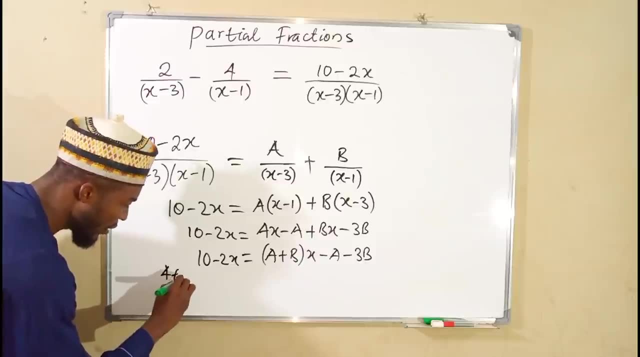 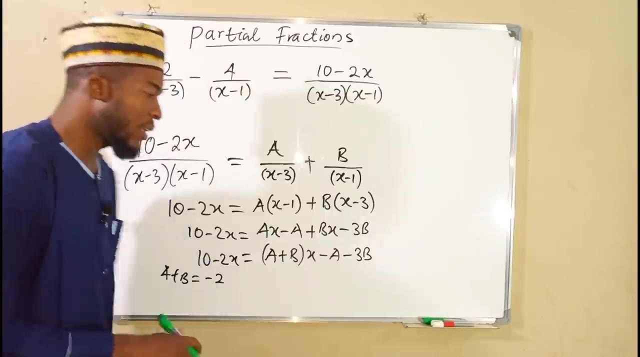 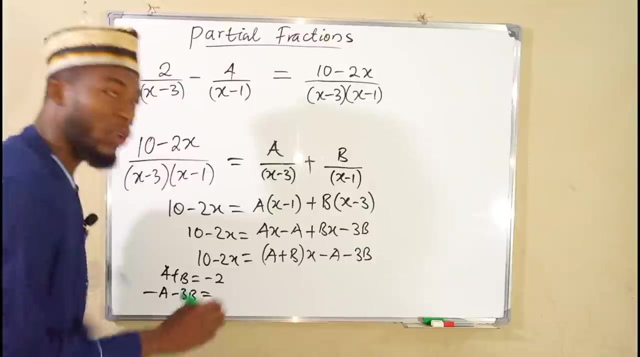 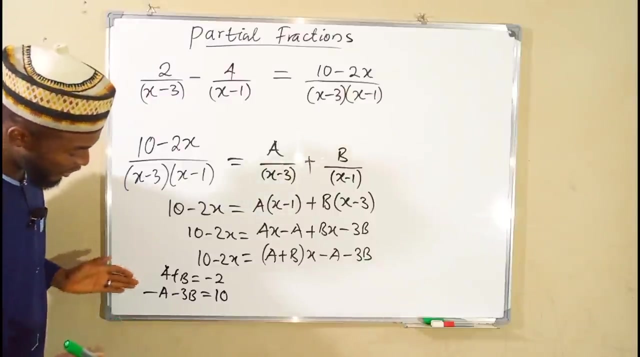 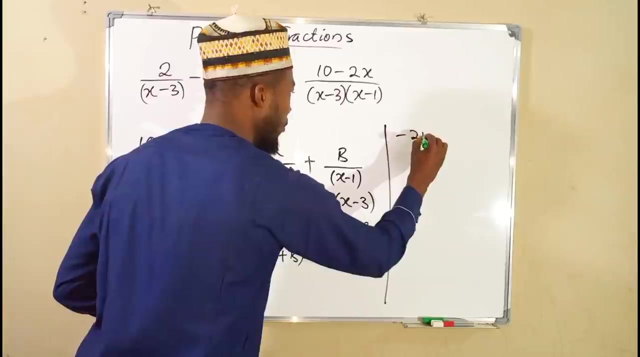 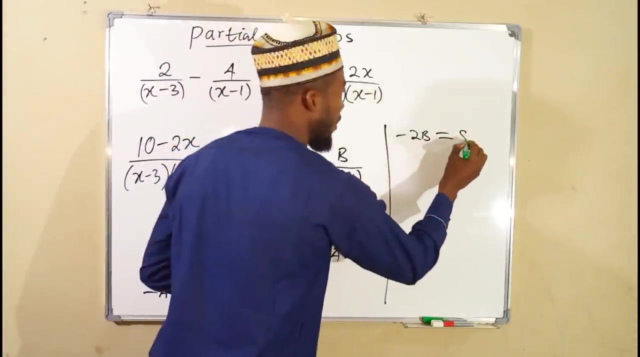 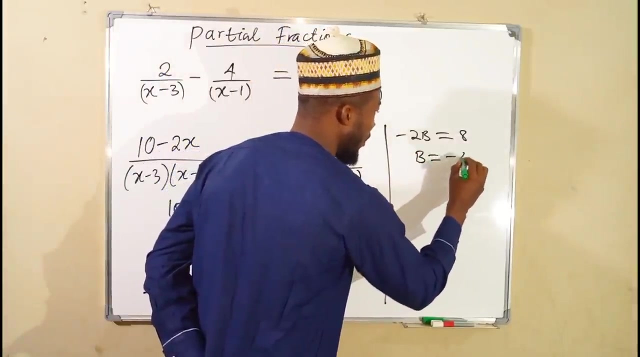 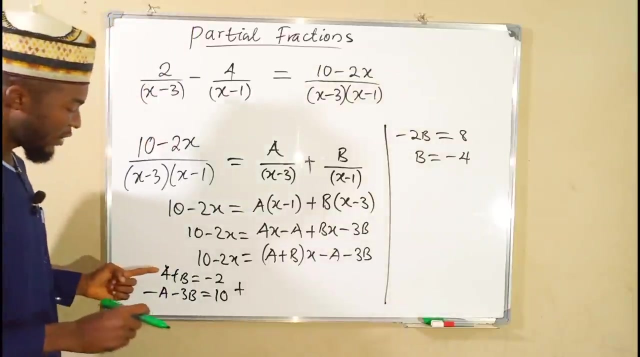 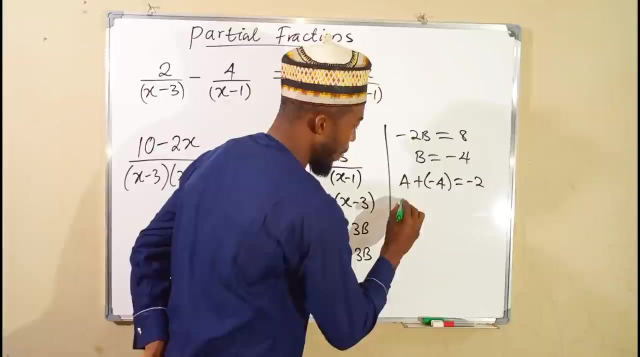 You can see the coefficient of x to the right is a plus b. The coefficient of x to the left is negative 2. We want to say a plus b is equal to negative 2. The constants to the right, we have negative a, negative 3b, negative a, negative 3b. This is equal to the constant to the left, which we have here as 10. You can see we can solve this by adding these two equations. We have a plus negative a is 0. Then b plus negative 3b is negative 2b. So we have negative 2b. This is equal to negative 2 plus 10 is 8. So we have 8 here. If you divide both sides by negative 2, you are going to obtain b equals negative 4. The value of b equal to negative 4. Either this equation or this. Then from here, you can see a plus b is equal to negative 2. But our b is now negative 4. So we have negative 4. This is equal to negative 2. a will be equal to negative 2 if this crosses over. 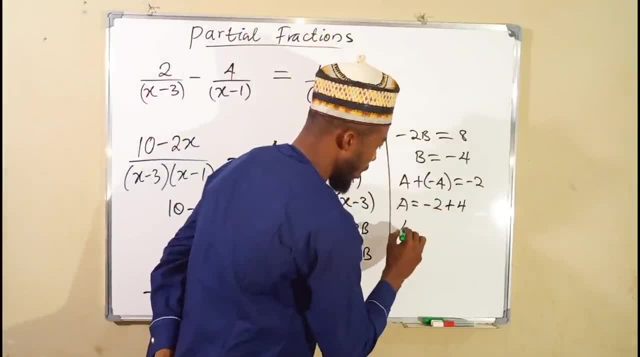 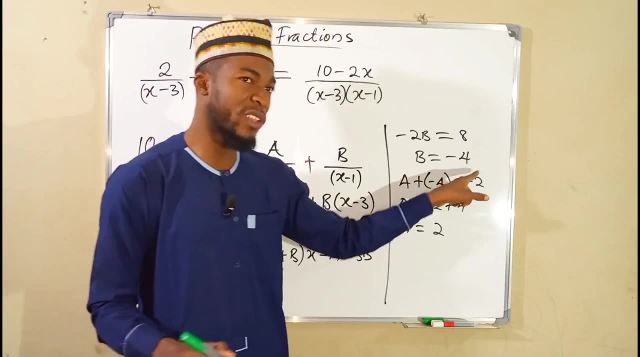 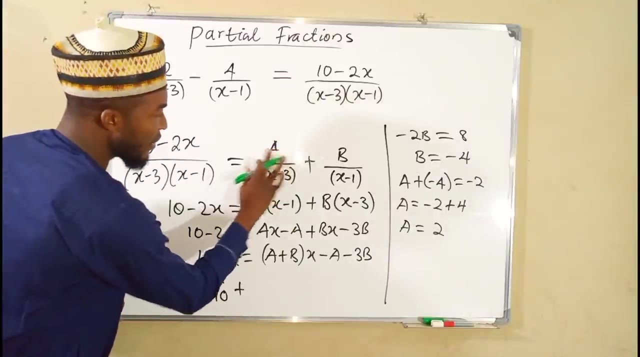 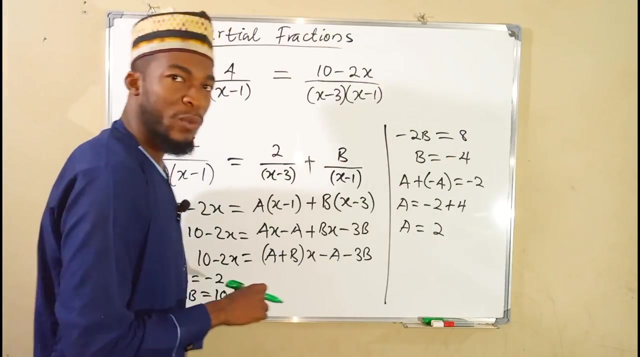 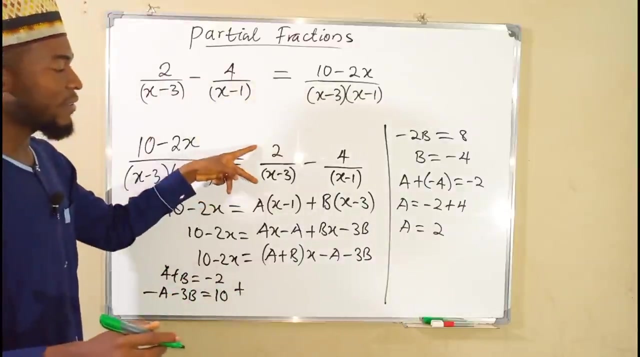 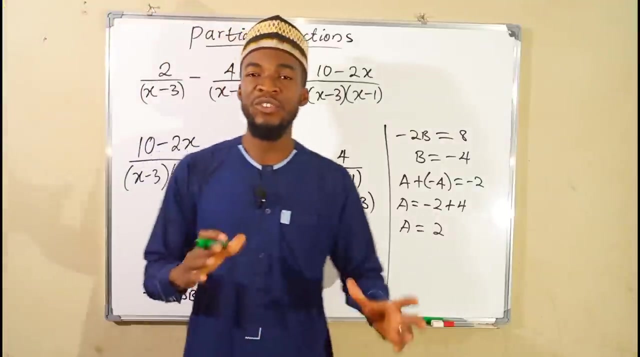 It becomes positive 4. And a will now be equal to positive 2. The constants of a and b are 2 and negative 4 respectively, which you can now substitute back to obtain your partial fractions. You can see here our a is equal to 2. You replace a with 2. And our b is negative 4. You replace b with negative 4. So we have negative 4 here. This becomes negative. And hence, these are our partial fractions that are exactly as the initial partial fractions. So this is just an introduction to partial fractions. Thank you for watching. Do have a nice day.